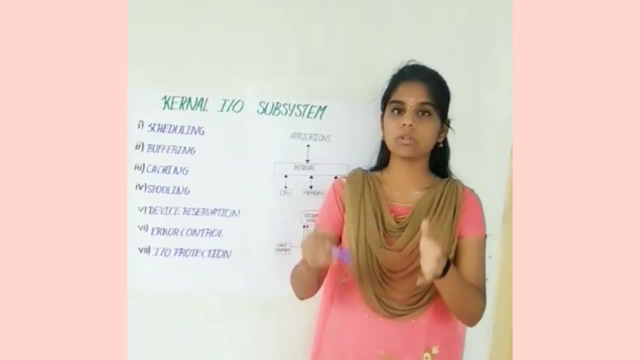 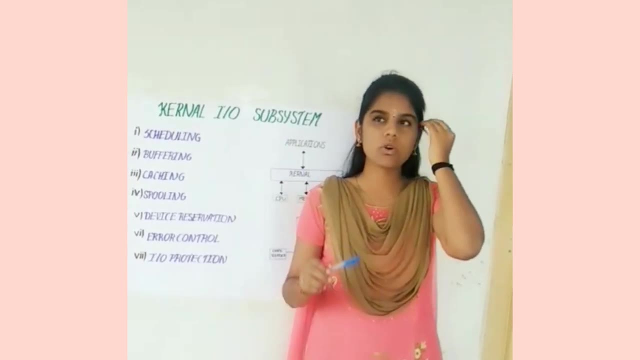 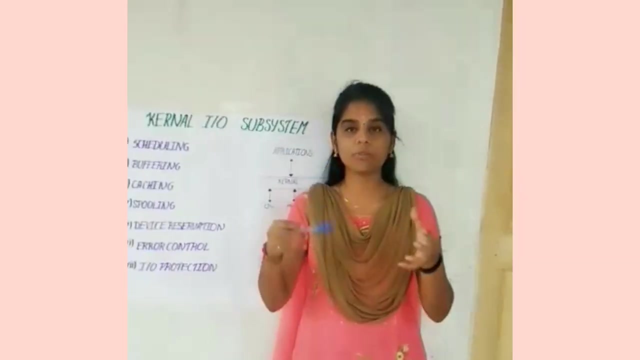 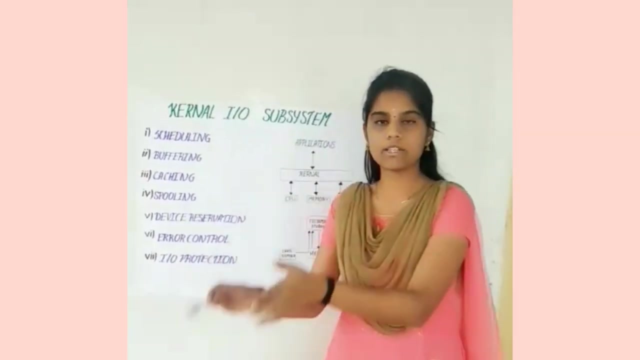 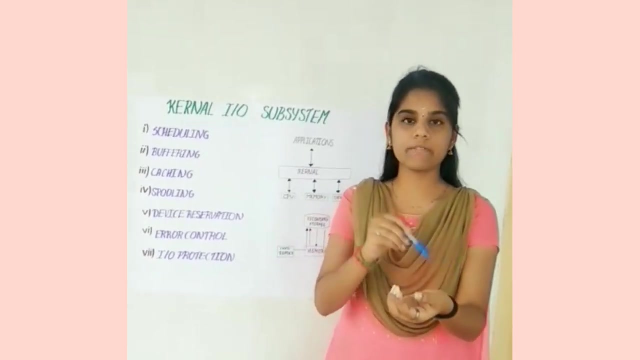 Ok. So Scheduling means in order to arrange the inputs, requests- and the outputs- is known as Scheduling. So arranging the orders, arranging the Arranging the system calls in a good manner is known as Scheduling. and Buffering means if it is a hardware and it is a software. means if you are transferring some data to one part to another part. in between these two devices there will be a storage space and the data will be stored here. 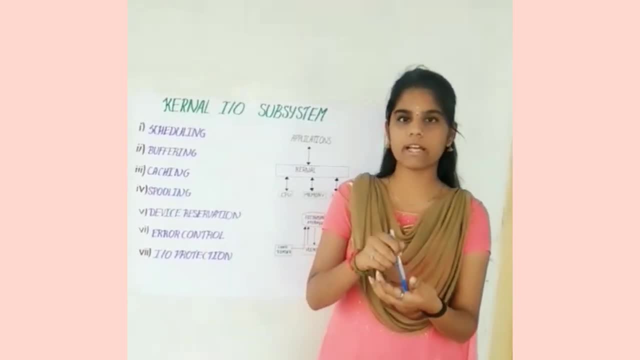 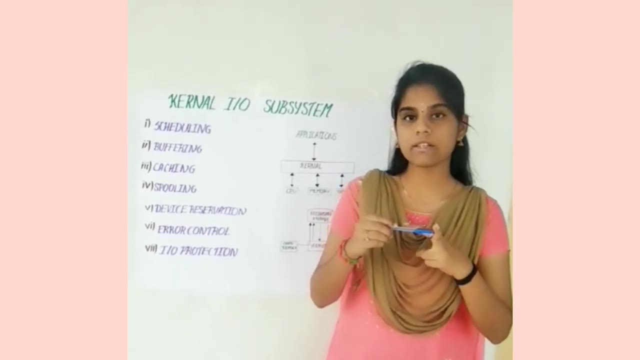 So you may have one question why we are storing the data here. So there are two reasons. The first reason is to cope with data, The second reason is to cope with the speed mismatch and the second reason is to cope with the data size mismatch. 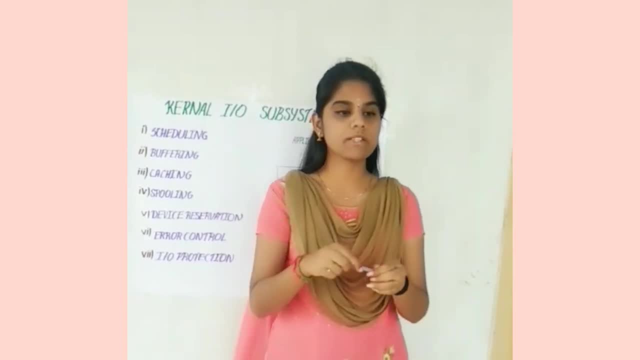 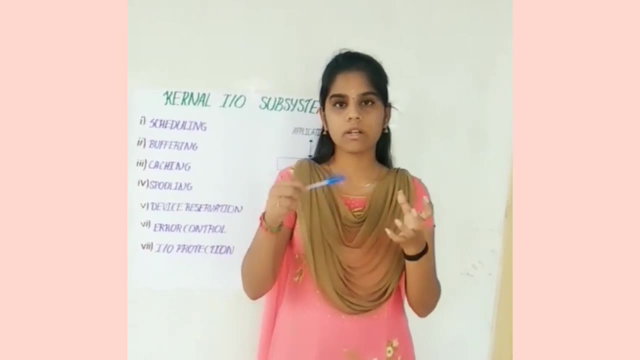 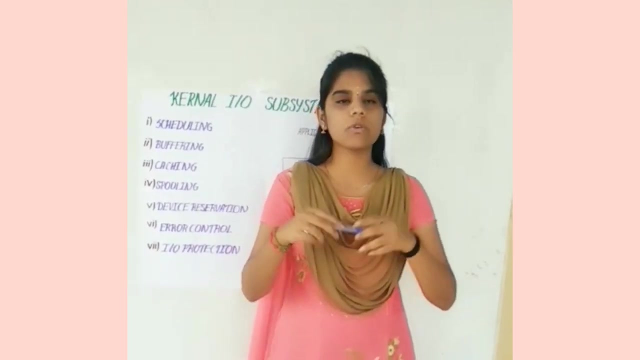 So cope with the data. speed mismatch means there are many inputs and there are many transfers and there are many system calls and if you have to transfer some data, there will be different data timings to transfer data. Ok, So you have to equalize the data. 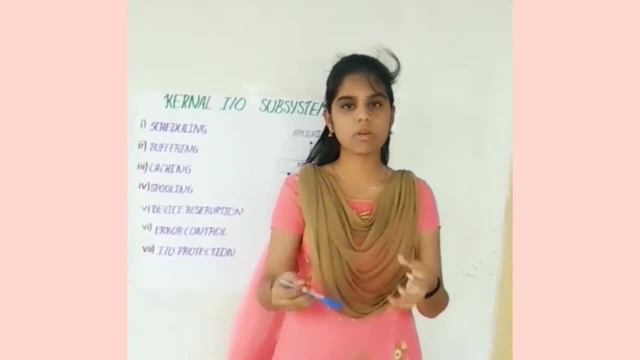 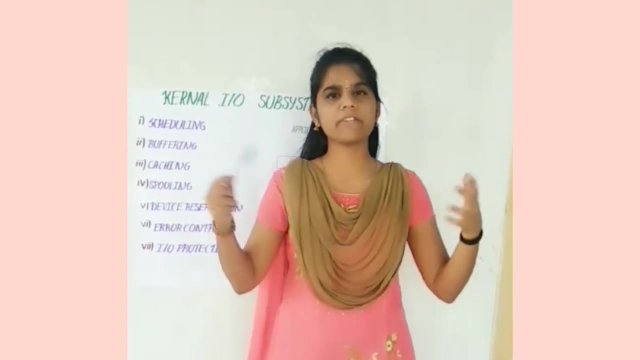 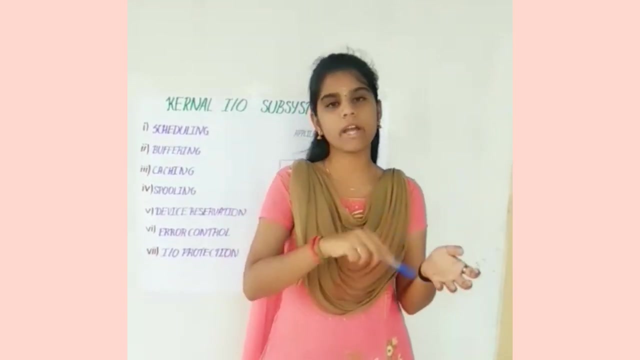 So this is known as Speed Mismatch And Data Size Mismatch means there are many different kinds of data with different sizes. There are not equal size data while transferring ok. So this is known as Cope with the Data Size Mismatch. 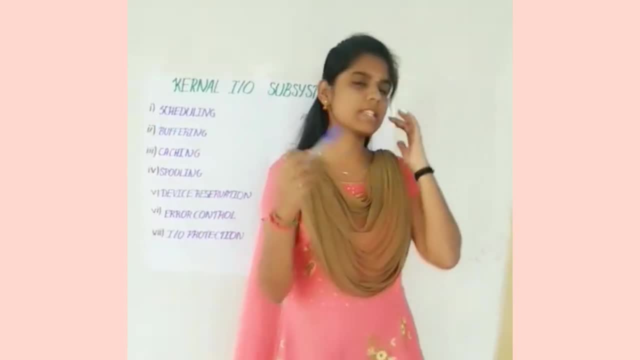 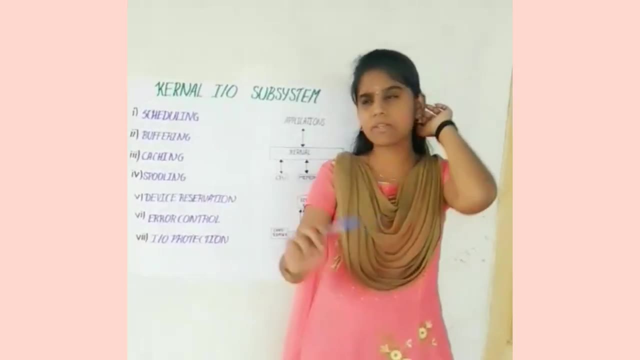 So to equalize this, we are using this Buffering. Buffer is nothing but a register. That's a temporary storage space, that's all. And Caching. Caching means there is a slight difference between Buffering and Caching. In Buffering, you are storing the original data. In Caching, you are storing the duplicate data of the original copy. That's all. This is a slight change, or slight difference between Buffering and Caching. Now we will be moving to the Spooling. 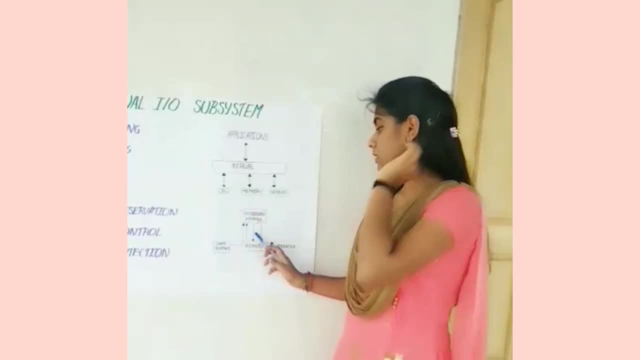 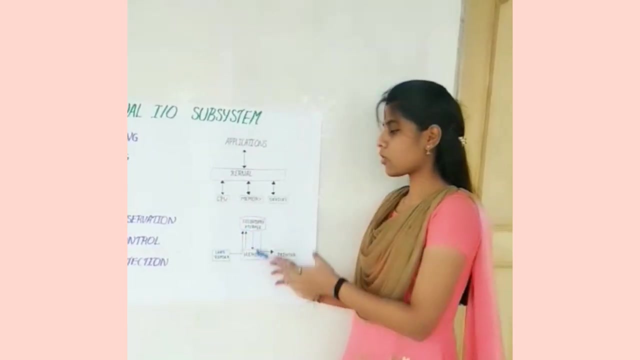 Spooling means this is Card Reader, this is Memory, this is Secondary Storage and this is Printer, ok. Ok, If the Printer wants to access data from Card Reader means the first. the Card Reader will sense the data through the Cache. 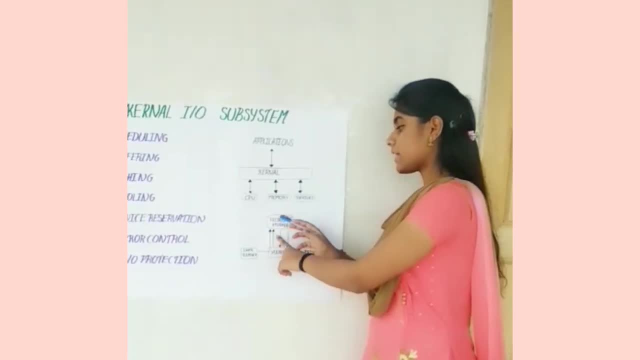 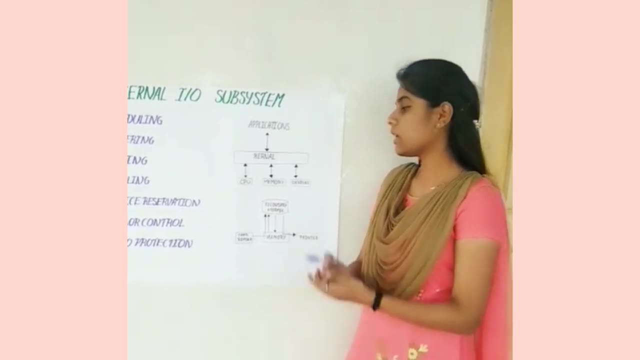 Ok, Ok, Ok, Ok, Ok, Ok, Ok. So you are storing the Secondary Storage and it will access the data here and sends to the Main Memory and the Main Memory will sense the data to the Printer. Ok, And again, it will store to the Secondary Storage Disk. 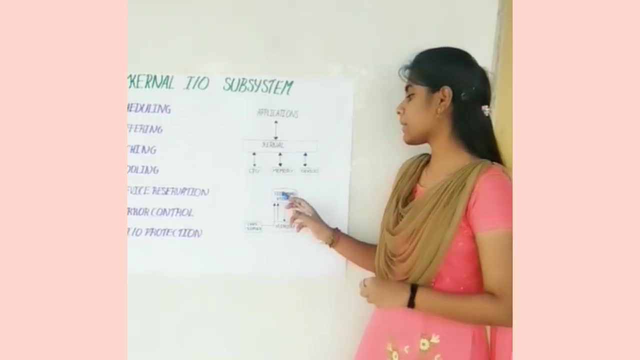 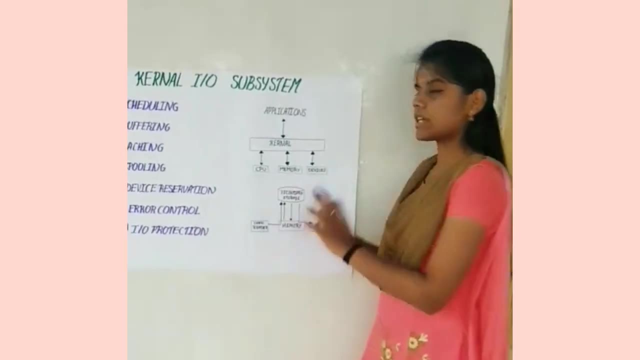 Whenever the Printer- or whatever may be the Output Disk- wants to access the data, the Printer will send the data. the Secondary Storage will send the data from Memory to Printer. That's all. This is known as Spooling. Spooling means. 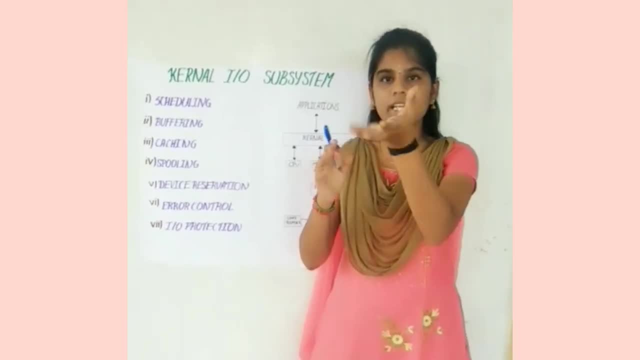 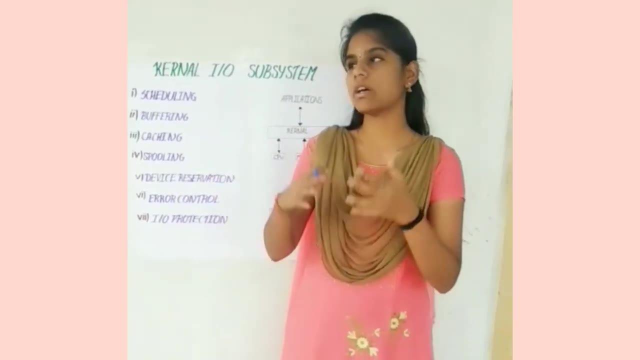 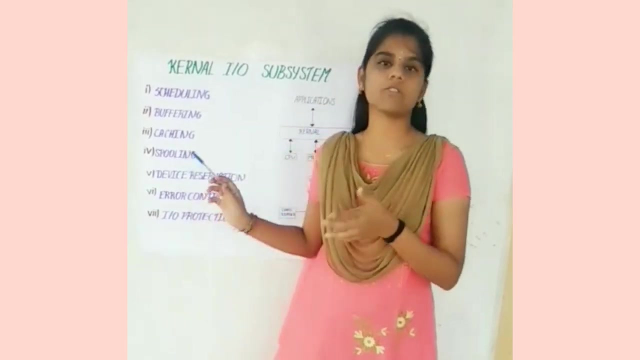 So using the data for a temporary time is known as pooling, And there is reservation. There is reservation means allocation and deallocation of data, is known as there is reservation. Error control: Error control means controlling the system. errors is known as error control. 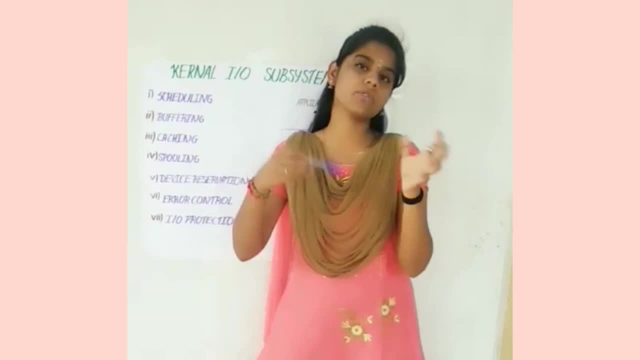 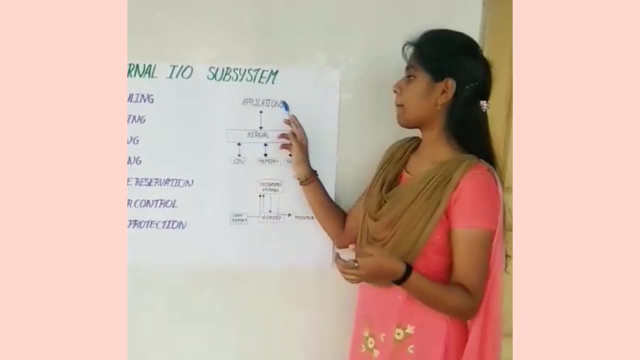 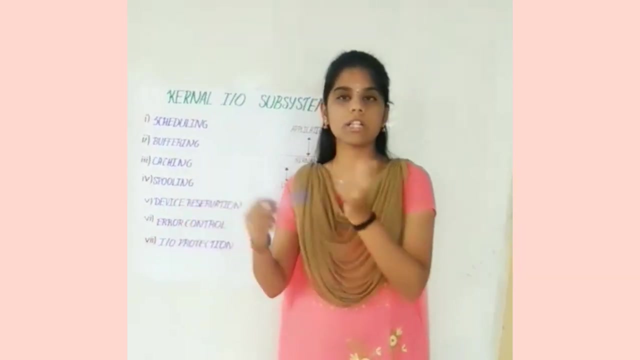 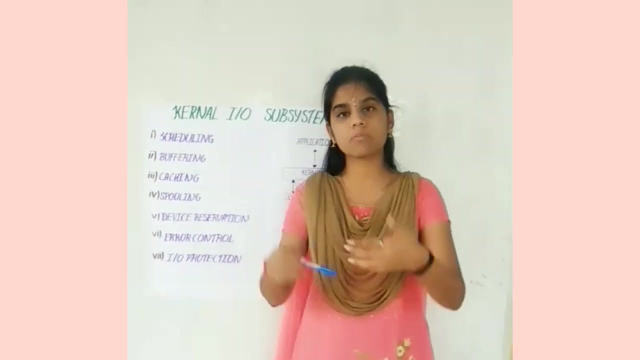 IO protection. The processor protects the IO using system call. System call means. in the earlier session of this video I explained what is system call. The application sends the request to the kernel. This request is known as system call. Okay, So, while using the system call, the processor protects the input device and output device. So that's all. The session is over. I will again explain. Once again explain the overall glance about this kernel IO subsystem. 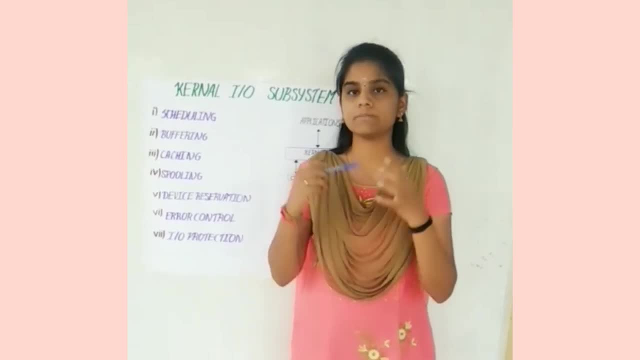 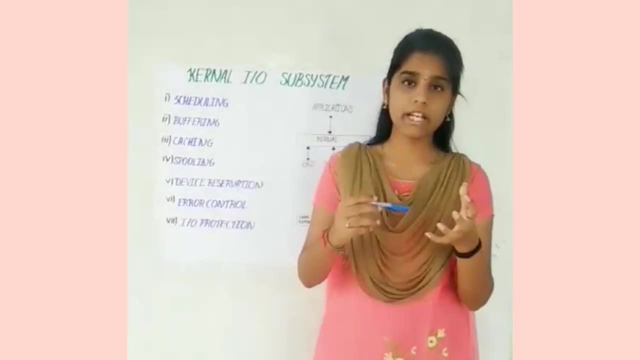 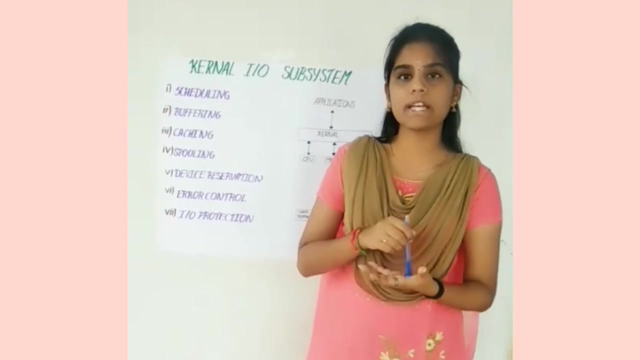 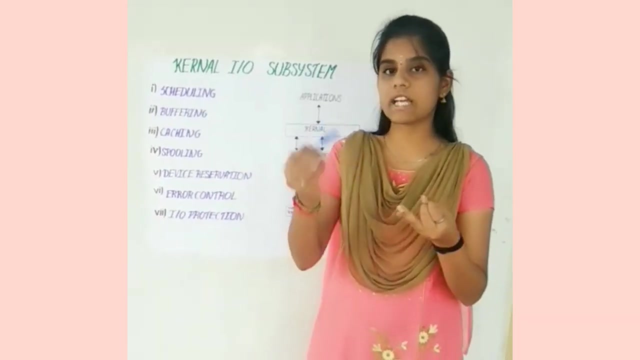 Kernel is the core part of IO. This is the operating system and it provides services to other parts of the OS. So scheduling means ordering the inputs in a good manner, is known as scheduling. Buffering means that's a temporary storage space. There are two reasons for buffering. The first reason is to cope with the speed mismatch and to cope with the data size mismatch. And caching means there is a slight change between the buffering and caching. In buffering you store the original data. In caching you store the original data. 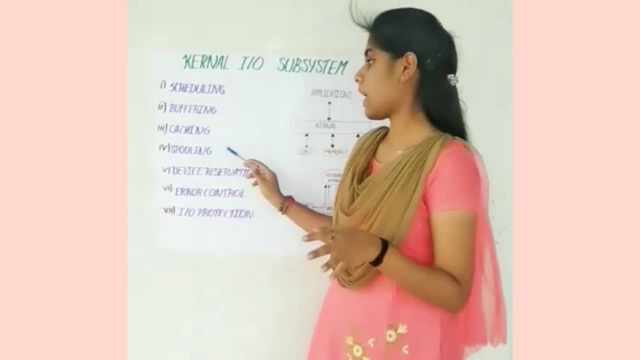 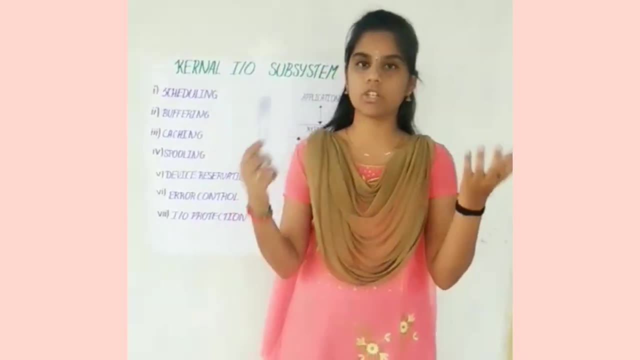 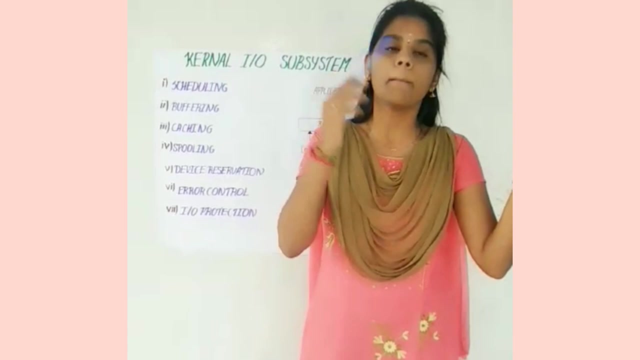 you store the duplicate data. that's all. and spooling means that's a temporary usage of data, is known as spooling, and Davis reservation means allocation and deallocation of data. error control means controlling the error system. error is known as error controlling. IO protection means using the processor and system for the input and output. Davis is all. 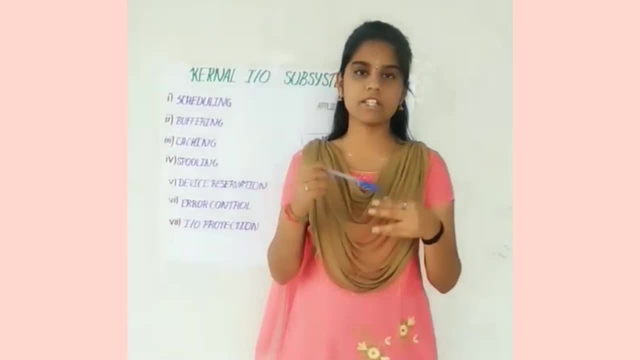 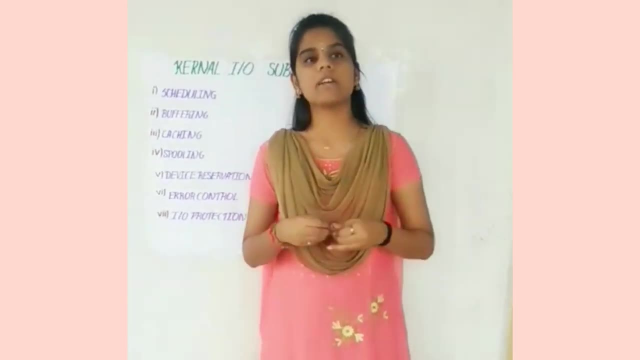 protected. so that's all. the session is over. I think the session will be useful for your study purpose, so thank you so much for listening this video completely, so we will meet at the next session. until shining of from Suganya.